but Latin America. It's Latin America. the trek up to northern Mexico or Argentina for the oldest barbecue tradition in the world, First stopping by Cuauhtémoc Moctezuma Brewery when you're old enough for a German-inspired Mexican beer. Rounding out your trip by finishing off in Buenos Aires, the Paris of the West. 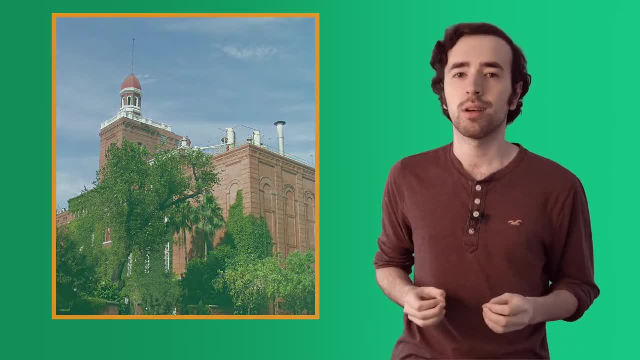 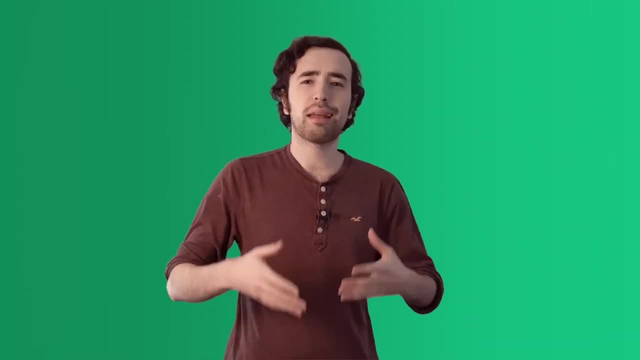 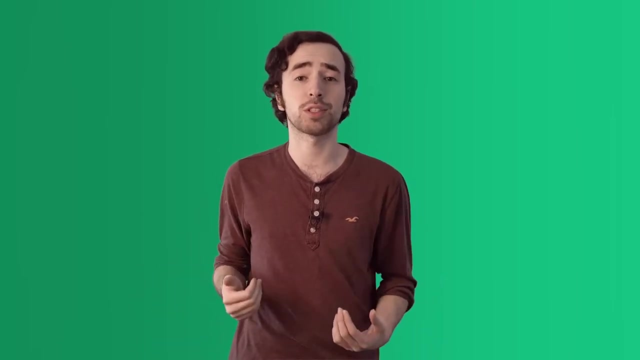 for European cuisine par excellence. Clearly, we've made some progress right Now. was that everything about Latin America? Absolutely not. For a teacher, a lesson is always a place not to complete an idea but to ignite curiosity in you, the student. So 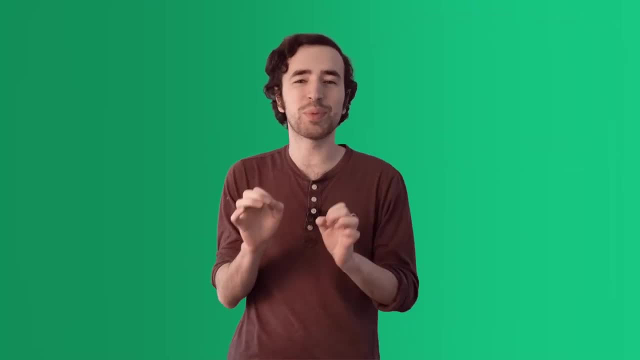 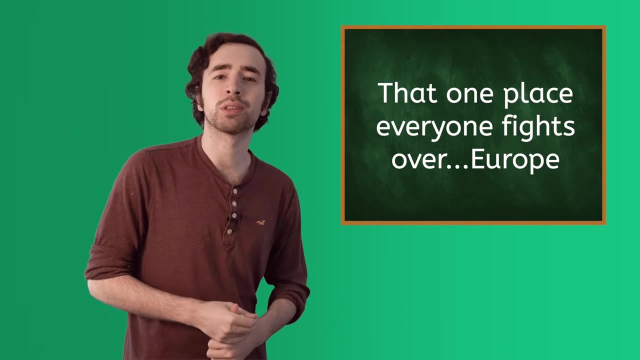 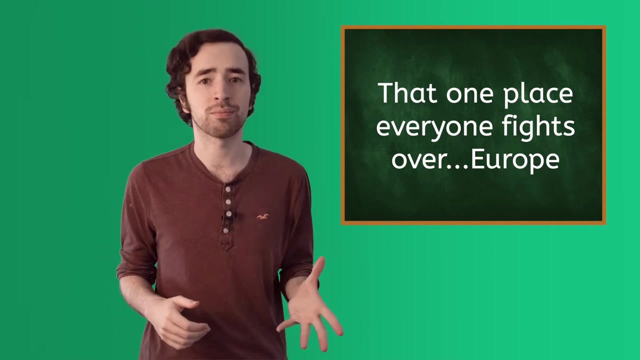 as long as you're always hungry to want to learn a little bit more. we've done our job. Now back to those explorers that came over to Latin America, all looking for their own little- Maybe not so little- piece of it. Remember where they were all from. That's right, Europe. When you 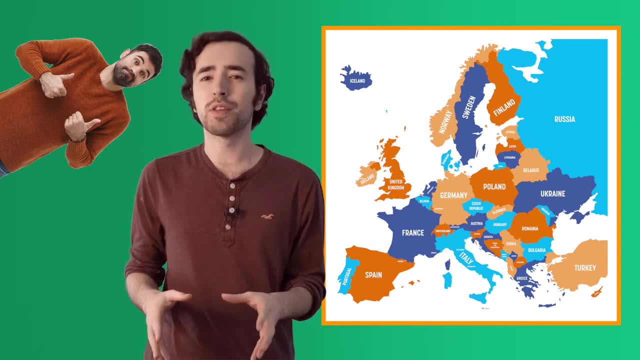 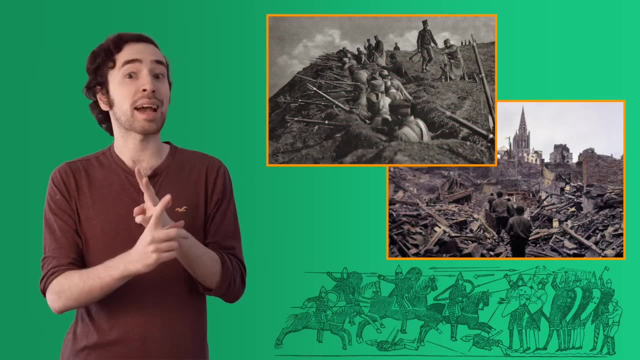 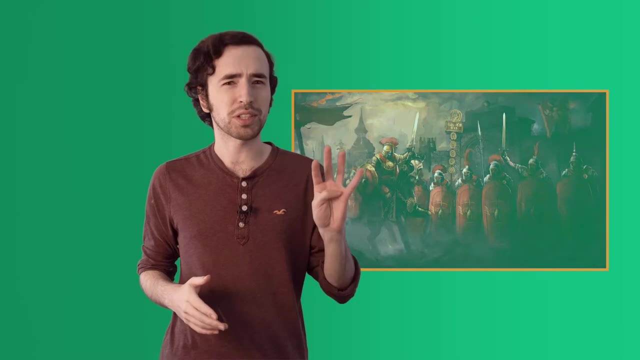 ask the average person about Europe, most, if not all, of them will mention one of three things: World War I, World War II or knights in castles. If they're smart, they might bring up the Roman Empire and talk about their legions. But do you notice a theme here? All the most common ideas. 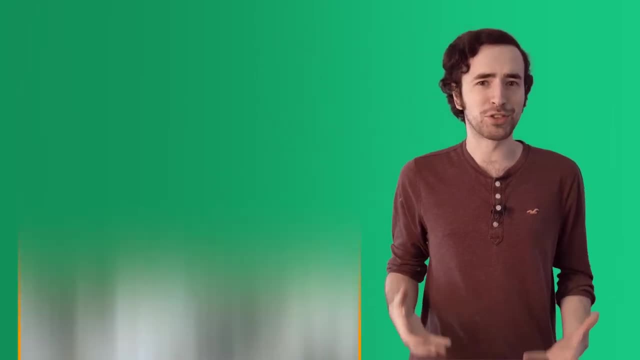 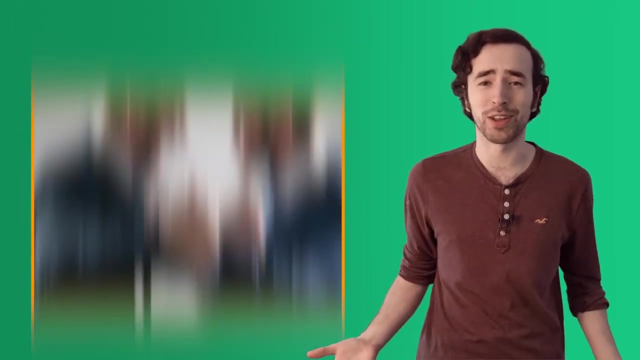 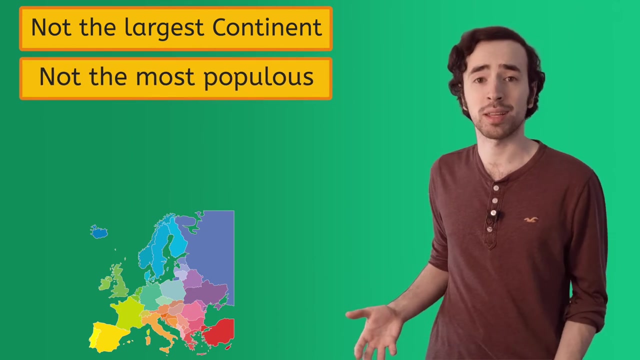 that people think of when they think of Europe have to do with war. Weird right. So why does everyone want to fight over Europe? At first glance it doesn't make much sense. It's not the biggest continent, It's not the most populated continent, It's never even been close. 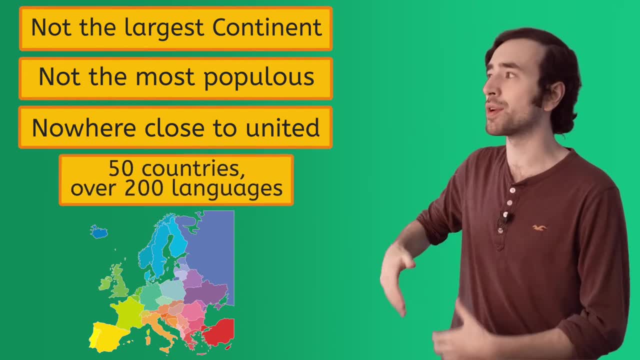 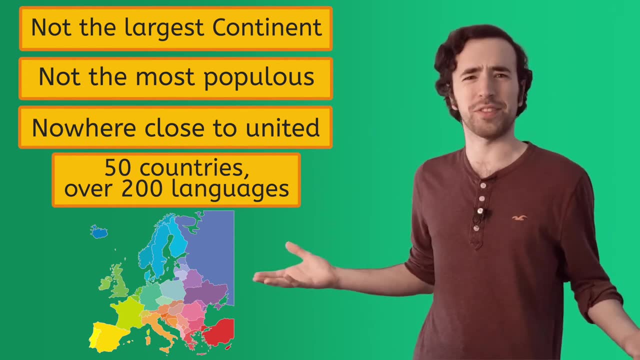 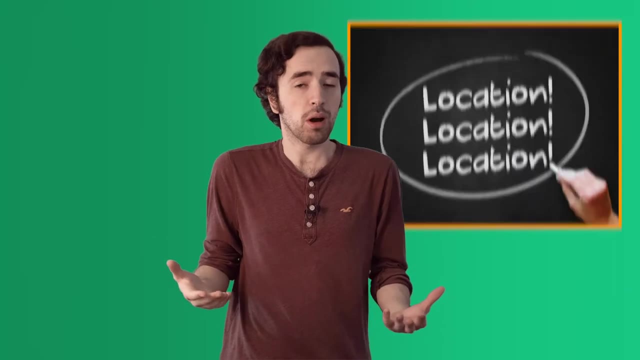 to being united in the past, as evidenced by the number of different countries or different languages. there, 24 official, over 200 spoken. So what? Who gives? Well, as a geographer, you have to remember that our study is about, among other things, 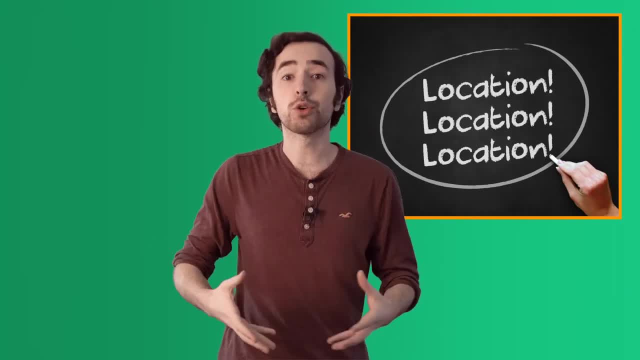 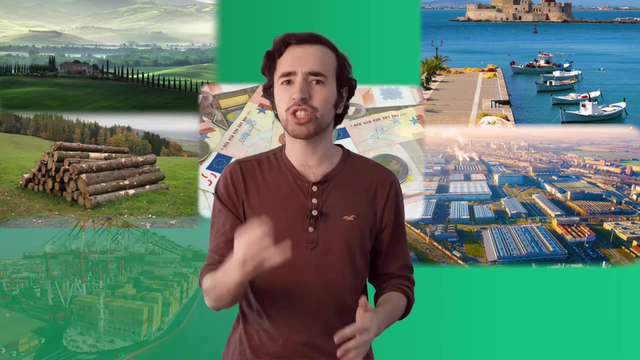 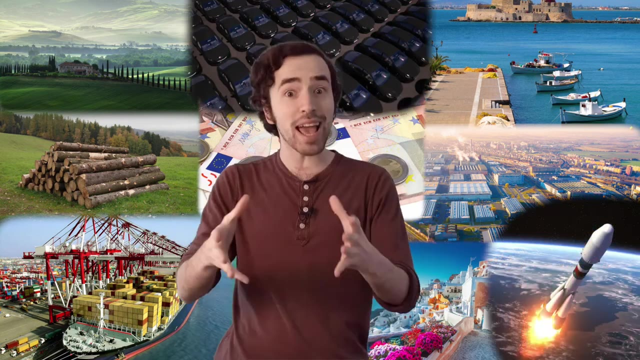 location, location, location. Europe's location makes it a prime spot for farming, fishing, logging, industry, banking, shipping and tourism. In addition to that, Europe also has among the first and the largest automotive and aerospace industries, and they're the largest exporter of.